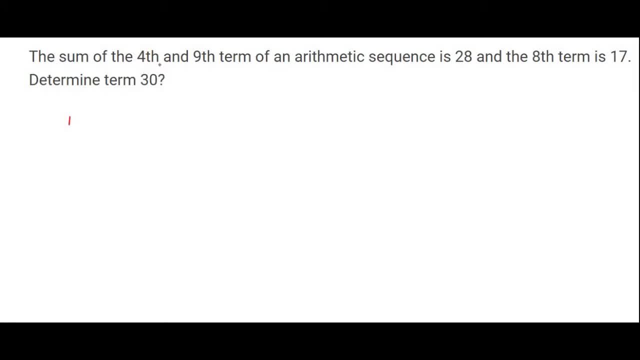 four terms. However, they're saying that the sum of only term 4 and term 9 is 28.. So what this actually means is term 4 plus term 9 is 28.. Then they also tell us that the eighth term is 17.. So 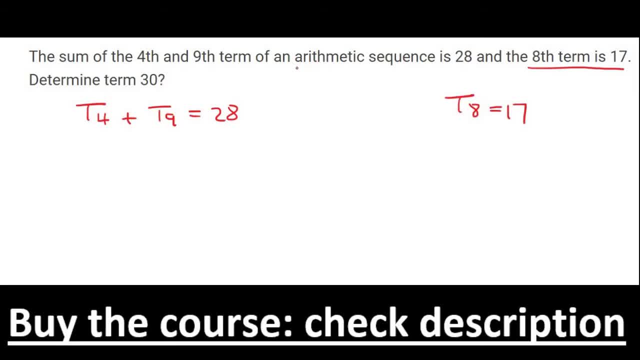 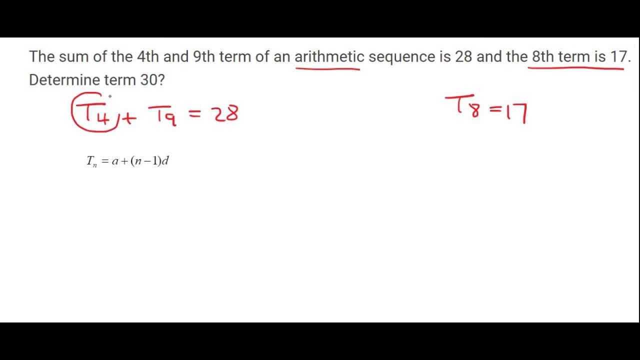 we can say: T8 is 17.. They tell us that it's an arithmetic sequence, and so we can use the following formula: And so in the place of term 4, we could say a plus 4 minus 1 times d plus. 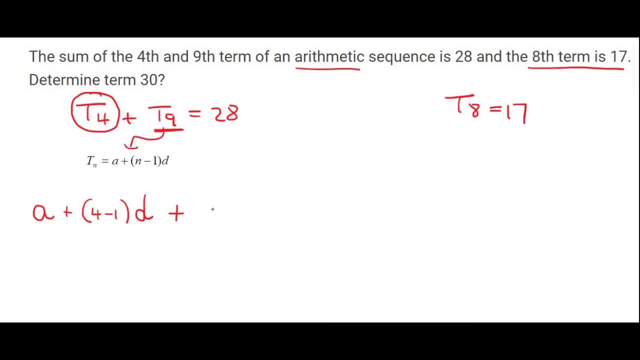 then again we can fill in term 9 using this formula, So that would be a plus 9 minus 1 times d, and that equals to 28.. We could then simplify a little bit so that would be a plus 3d plus a plus 8d is 28.. 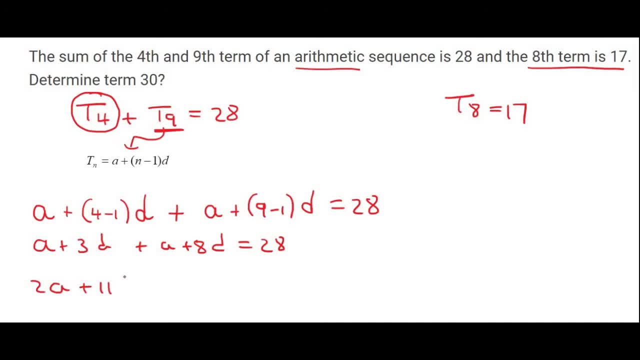 Further simplification means that 2a plus 11d would be 28.. We can't go any further because we have two unknowns. We now go to our other equation, which tells us that term 8 is equal to 17, and so that means 17 is going to be equal to a plus 8 minus 1 times d. 17 would then be equal. 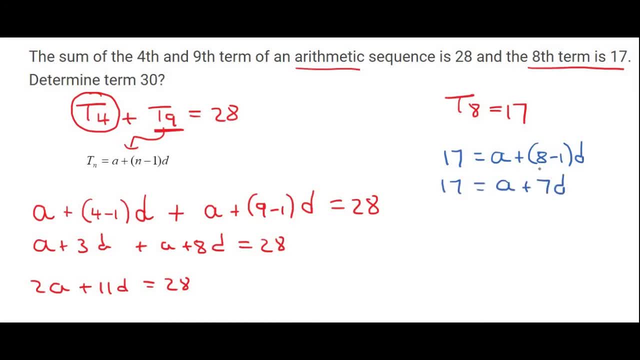 to a plus 7d. We now have two equations, two unknowns. There are various ways that you could solve this. What I'm going to do is I'm going to use this equation and get a alone, and so that would be: a is equal to 17 minus 7d, and I'm going to plug that into the other formula. 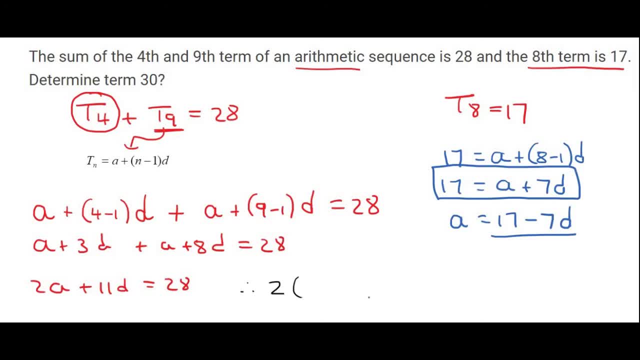 And so that means we'll have 2, and then in bracket I'm going to replace the a with 17 minus 7d. I hope you guys can see I'm plugging into this equation: plus 11d is equal to 28.. 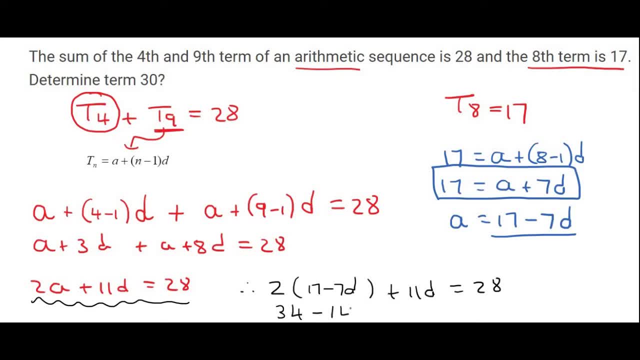 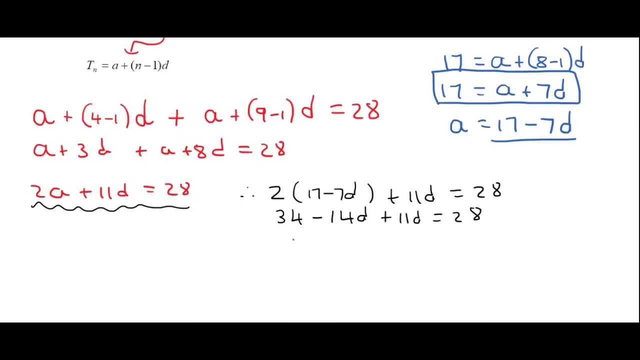 We then multiply the two in and that will be: 34 minus 14d plus 11d is equal to 28.. And then simplify a little bit. That's going to be: 34 minus 3d is equal to 28.. I'm going to take the. 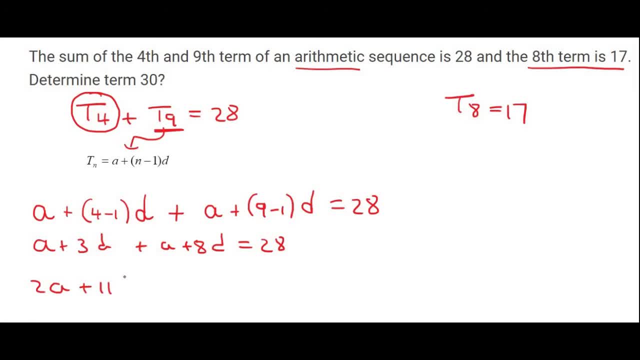 Further simplification means that 2a plus 11d would be 28.. We can't go any further because we have two unknowns. We now go to our other equation, which tells us that term 8 is equal to 17, and so that means 17 is going to be equal to a plus 8 minus 1 times d. 17 would then be equal. 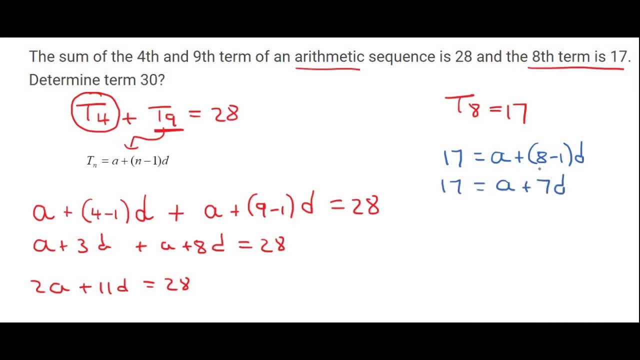 to a plus 7d. We now have two equations, two unknowns. There are various ways that you could solve this. What I'm going to do is I'm going to use this equation and get a alone, and so. So that would be: a is equal to 17 minus 7d. 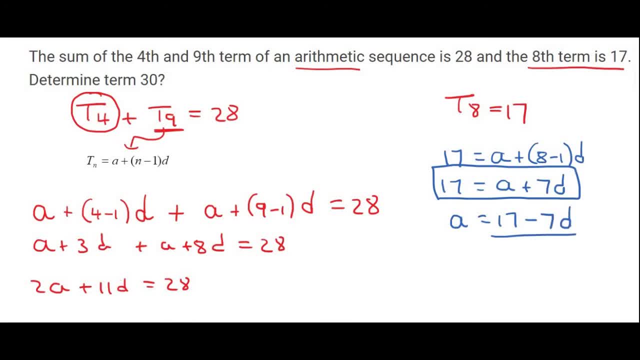 And I'm going to plug that into the other formula, And so that means we'll have 2.. And then in bracket I'm going to replace the a with 17 minus 7d. I hope you guys can see I'm plugging into this equation. 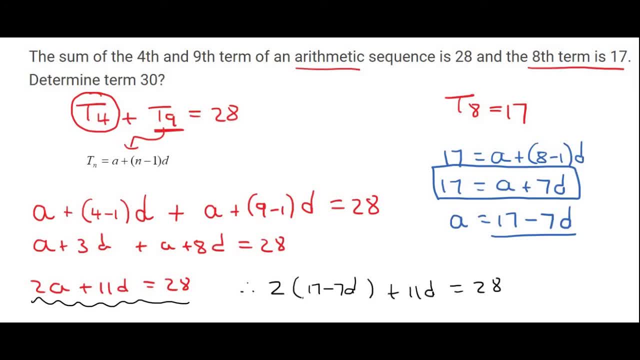 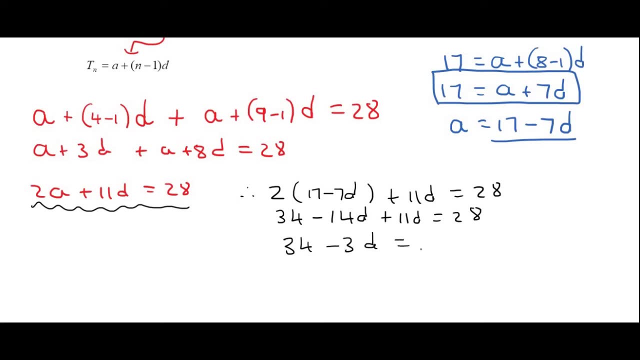 Plus 11d is equal to 28.. We then multiply the 2 in and that will be 34 minus 14d plus 11d is equal to 28.. And then simplify a little bit. That's going to be: 34 minus 3d is equal to 28.. 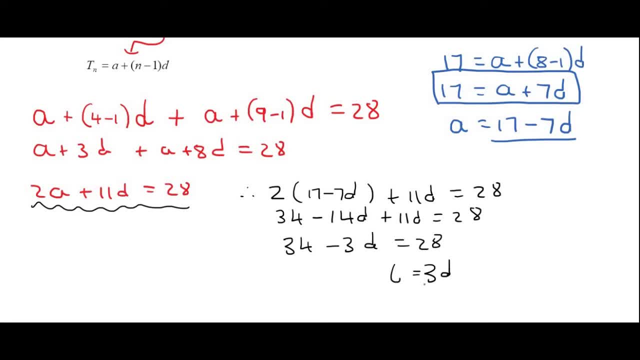 I'm going to take the 3d to the right, And on the left we'd be left with 6. And so this means that d is 2.. We can then plug that answer into here, for example, And so we would find that a is equal to 17 minus 7 times 2.. 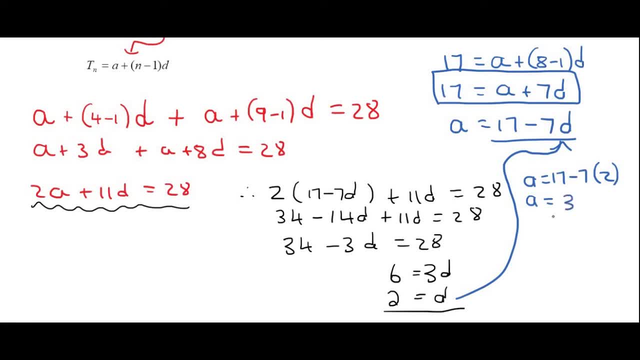 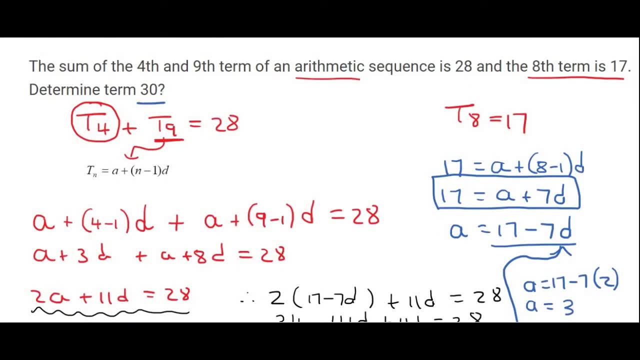 And so a. So a is going to be 17 minus 14. And so a is 3.. So we now have a and we have d. However, this question says: determine term 30. And so that's very easy now, because now to find term 30,. 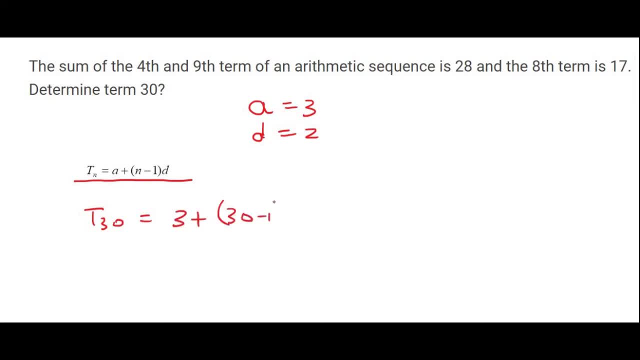 we can just say a, which is 3, plus 30, minus 1 times by d, which is 2.. Go ahead, type this all in on the calculator And you should get a final answer of 61.. And you should get a final answer of 61.. 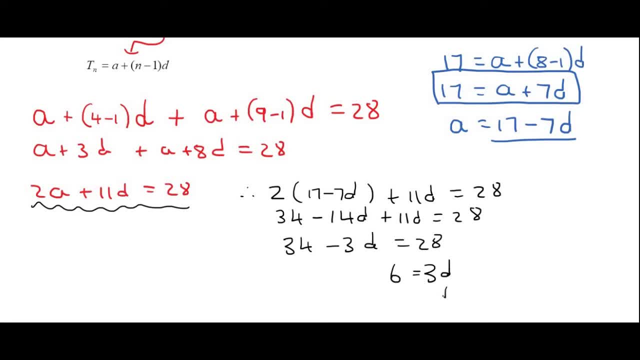 3d to the right and on the left would be left with 6, and so this means that d is 2.. We can then plug that answer into here, for example: And so we would find that a is equal to 17 minus 7 times 2, and so